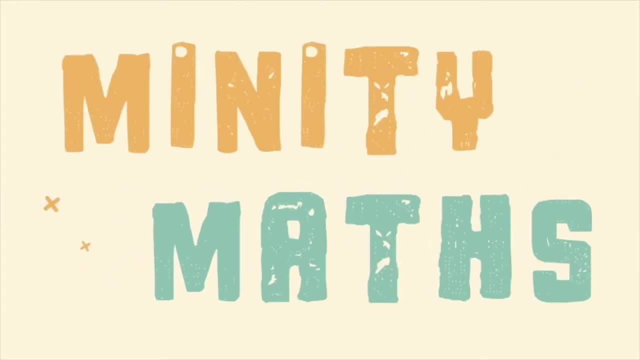 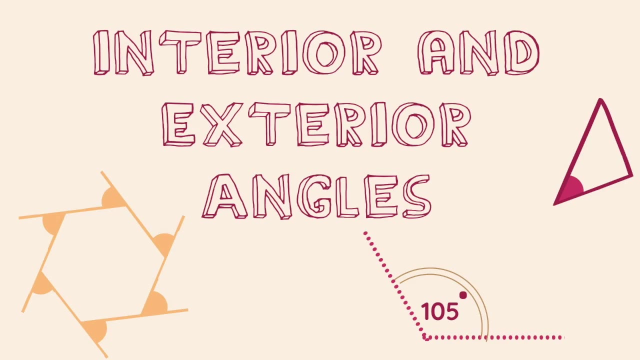 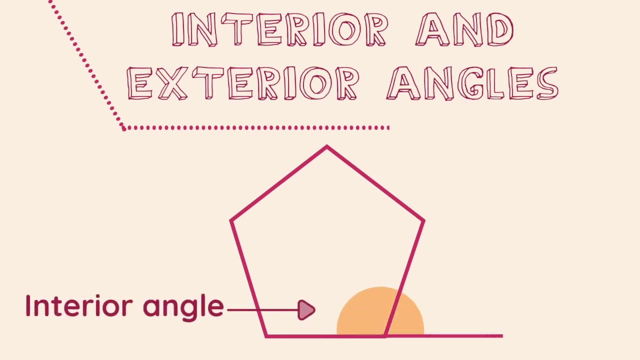 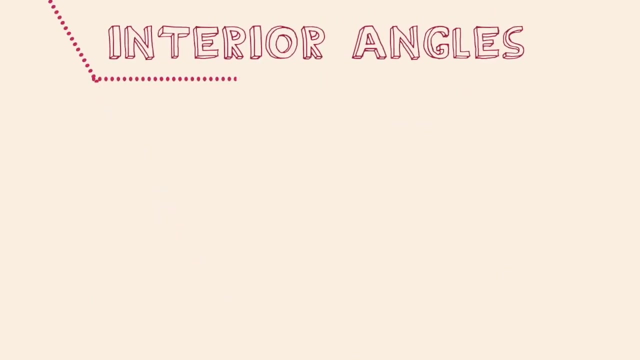 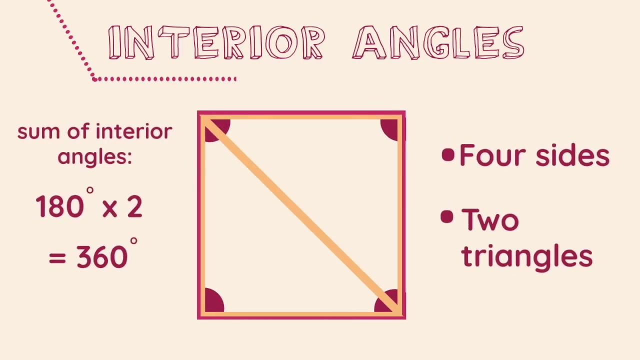 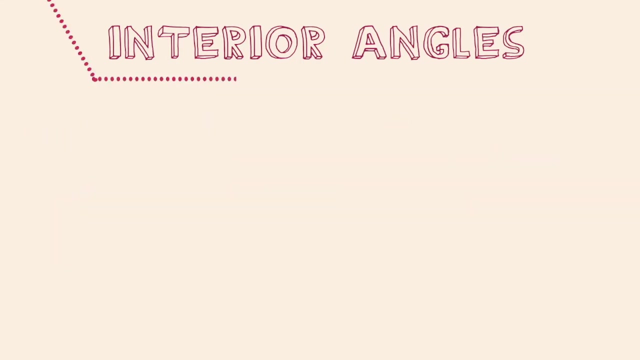 Interior and Exterior Angles. The first and most important thing to note is that the interior angles of a triangle will always add up to 180 degrees. Here we have a square. Notice that we can fit two triangles in the square. Therefore, the interior angles will equal two lots of 180 degrees. 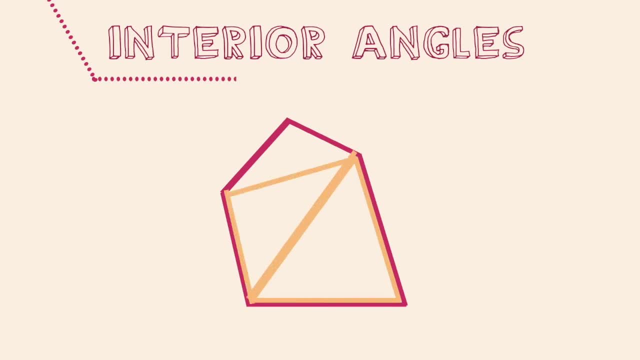 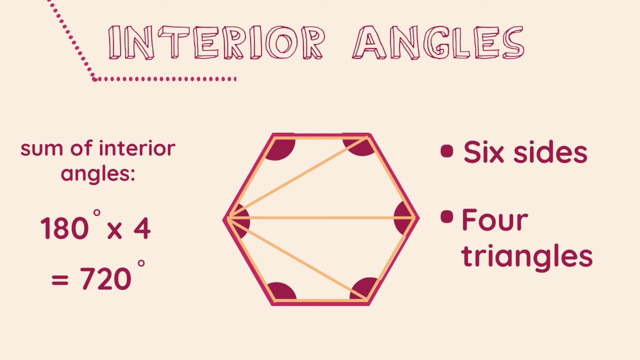 Next we have an irregular pentagon in which we can fit three triangles inside. Therefore, the interior angles will be equal to three lots of 180 degrees. Here we have a hexagon which can fit four triangles inside, So the interior angles will be equal to four lots of 180 degrees, as there are four triangles inside. 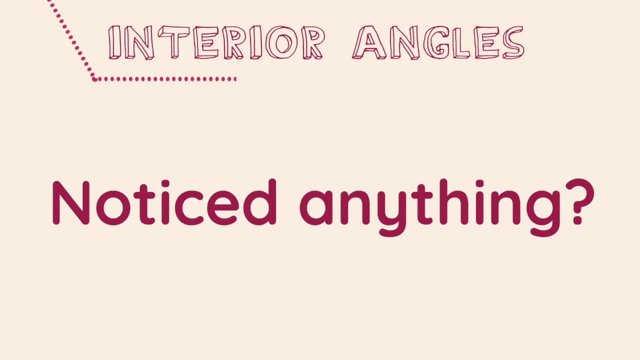 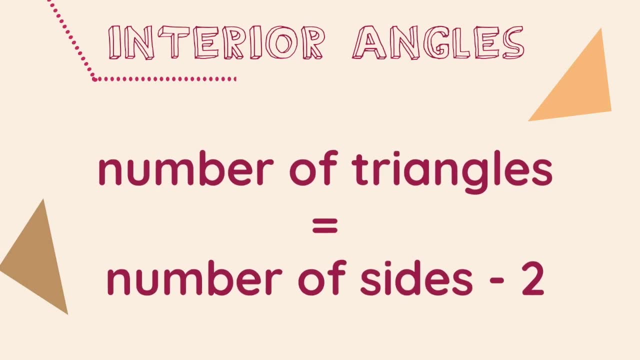 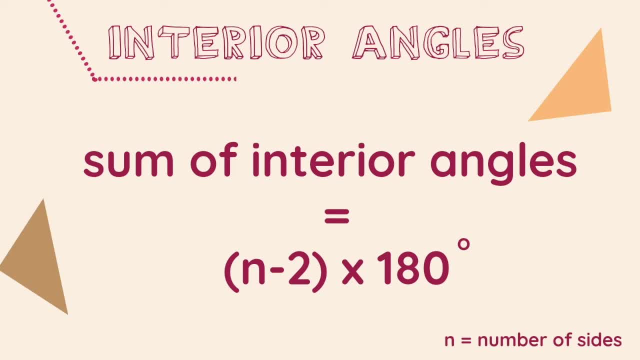 number of sides. So now we can create a formula which we can use for any polygon to find the sum of the interior angles. N is the number of sides. Take away two, and this gives us how many triangles can fit inside the polygon. We then times this by 180.. 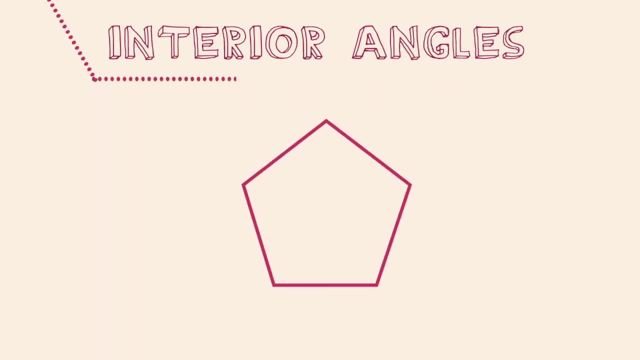 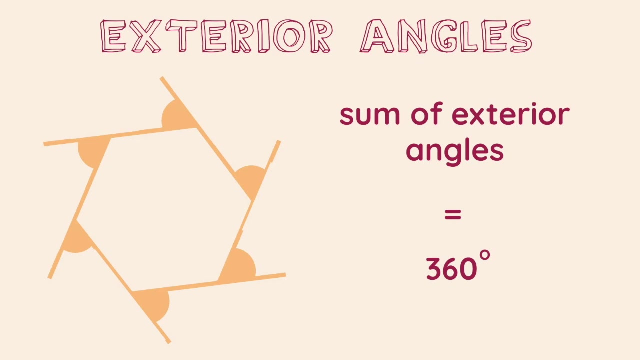 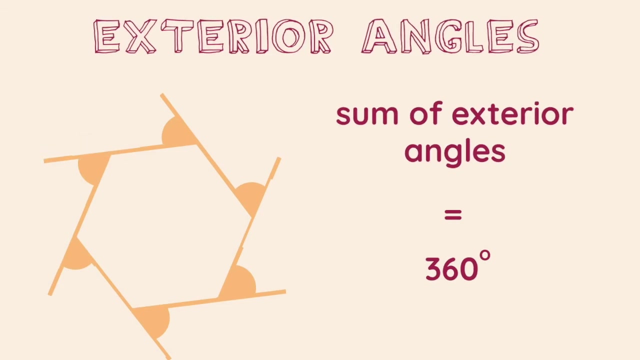 Exterior Angles- Exterior Angles. Have a look at this example. From this we can also calculate each interior angle by dividing your answer by the number of angles or sides. Now we are looking at exterior angles. The exterior angles of any polygon will always add up to 360 degrees.